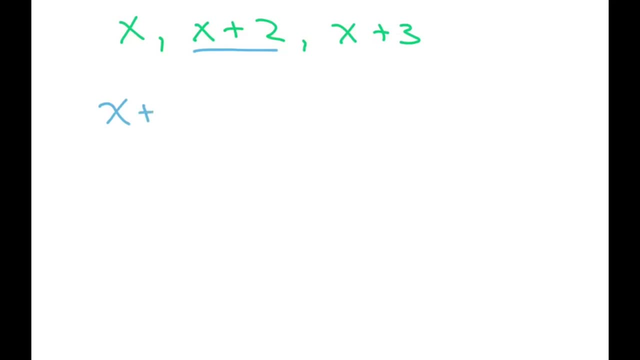 my current term and divide it by my previous term. That's your common ratio, And I'm going to do this one as well- My current term. divide it by my previous term, which is I x plus 2, and that gives me r, And then I'm going to set it up as a system of equations. 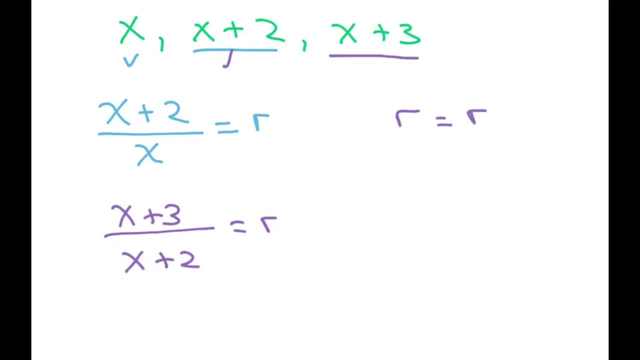 So we have r equals r. So I have x plus 2 over x equals x plus 3 over x plus 2.. Now we can cross, multiply and we'll get x squared. Show our work a little bit. We'll get x plus 2, we're crossing these two squared equals. 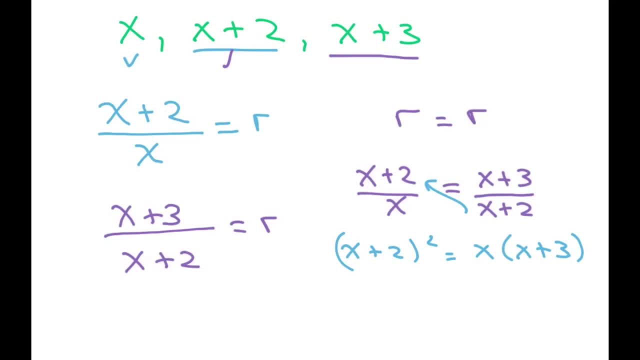 x times x plus 3.. So this is x squared plus 4x plus 4 equals x squared plus 3x. Now what happens is these two cancel. If I subtract the 3x and subtract 3x here, I'm going to. 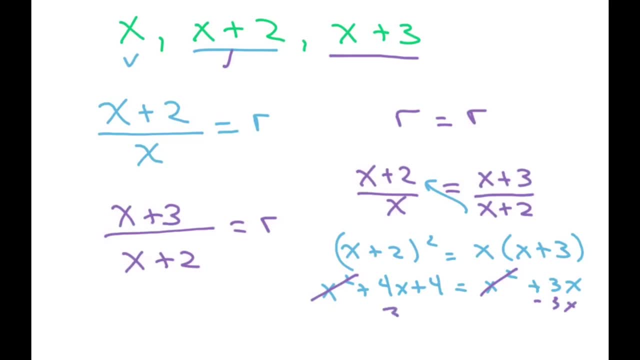 get 4x minus 3x is just x, And I'm going to subtract the 4. So x is negative 4. And if you want, you could plug in negative 4, and that's all we had to do, basically, is find our x. But 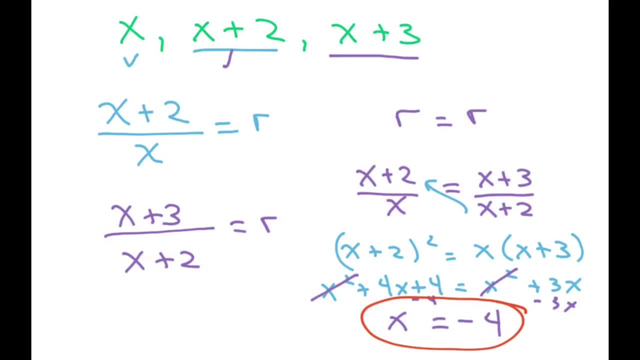 you can plug it in and see if it works. If I plug in my negative 4 here, I get negative 4.. Plug in negative 4 in this one, I'm going to get negative 2.. And I plug in negative 4 here, I get negative 1.. Or I get positive 1, actually right. Negative 4, I get negative. 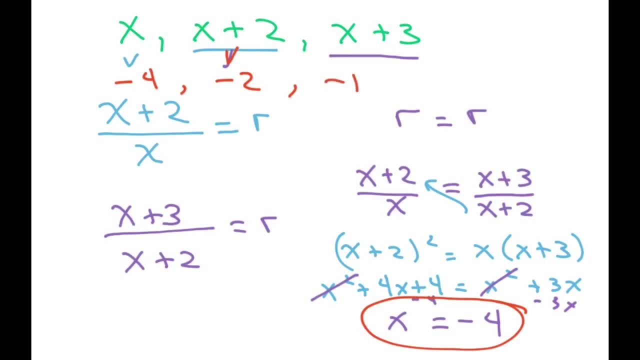 1.. All right, So basically, on this case, my common ratio would be 1 half, But that's not what we're looking for. We were looking for our x. That's all, Thank you, Have a nice day. Bye-bye.